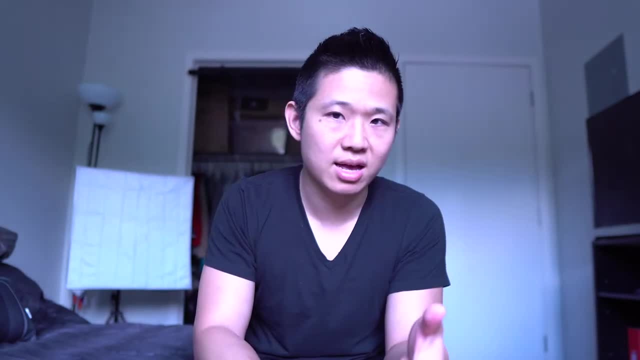 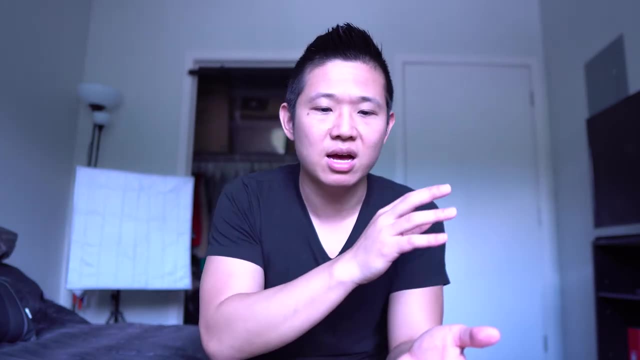 questions about: should i learn coding, should i learn excel, should i learn a sequel, should i learn all these different type of technical, pure technical skills and, i think, a lot of emphasis. maybe i haven't really done a good job of it, uh, granted, the technical stuff is great. 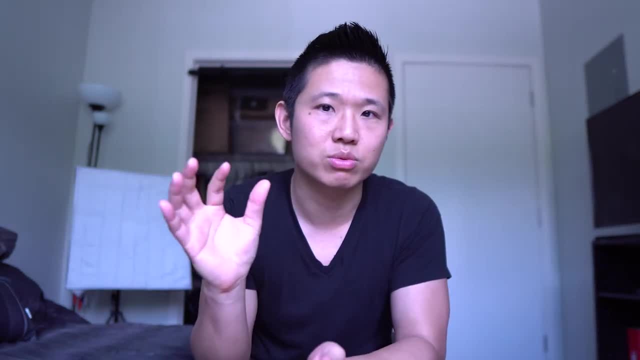 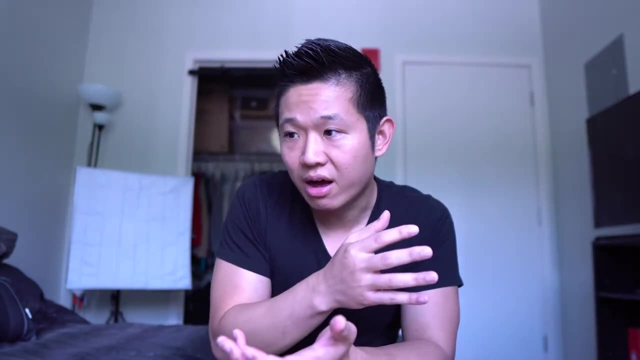 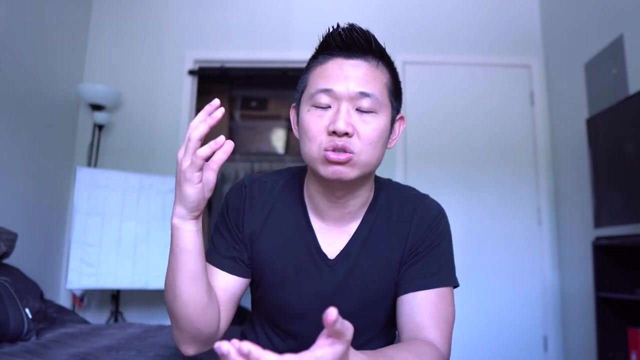 there is a whole other side of informatics that's really, really important, and there are, and i think in the next couple of videos i'm going to try and talk about a variety of these things, but today i want to talk about some of the project management principles within informatics. project management: 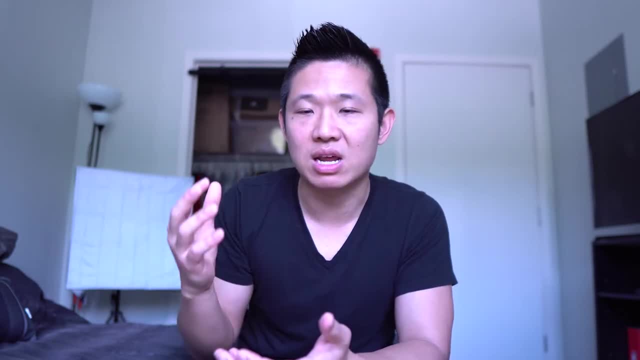 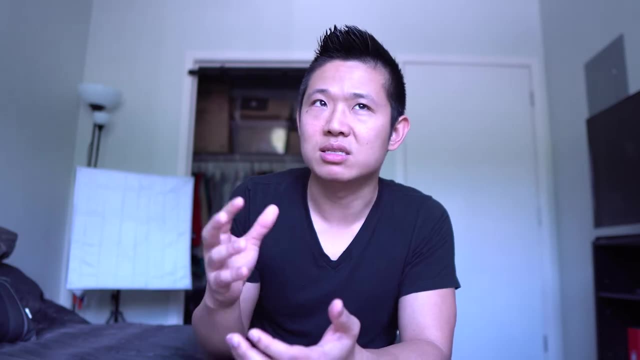 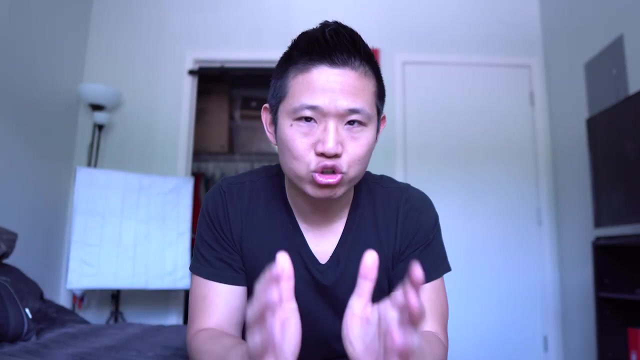 is super key in succeeding in this field, and i think it really needs to be talked about because a lot of it is also involving your soft skills. i don't really know where this topic today will fall under, but let's just get right down to it. so let's talk about the triple. 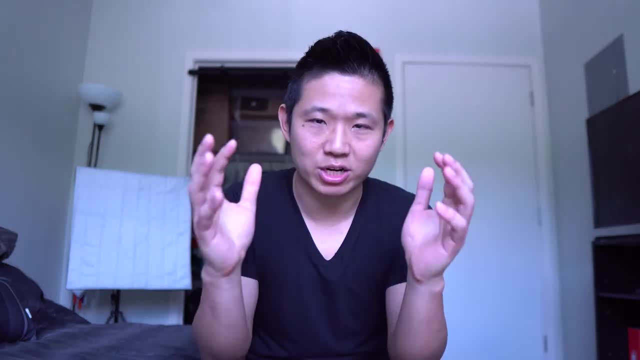 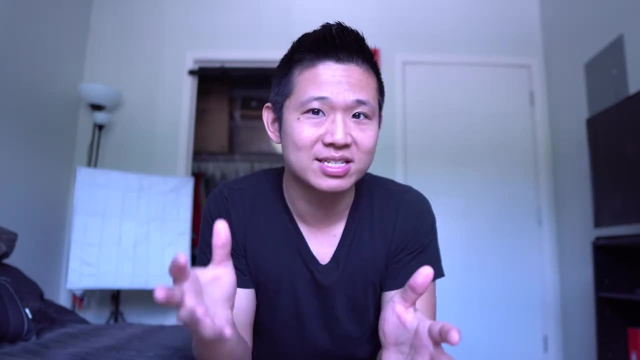 constraint and let's. i'm gonna go through some of the basics. i'm gonna try my best to make this uh video very brief, because i have so much to say about this. i can probably talk about this for days, like i am now just going off on some random tangent. anyways, i'm gonna try to get to the 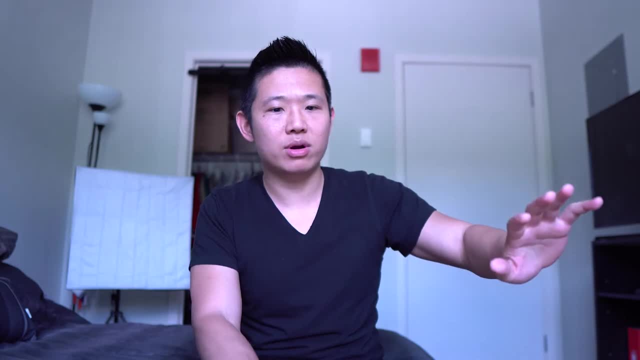 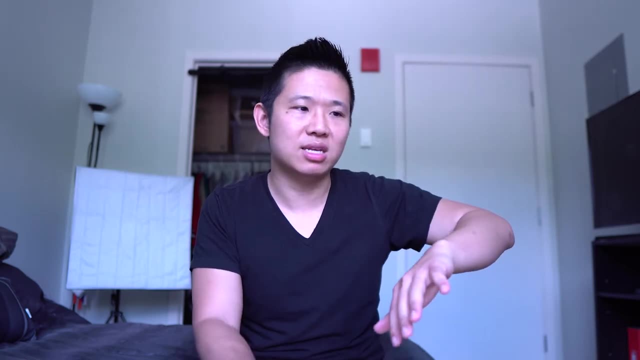 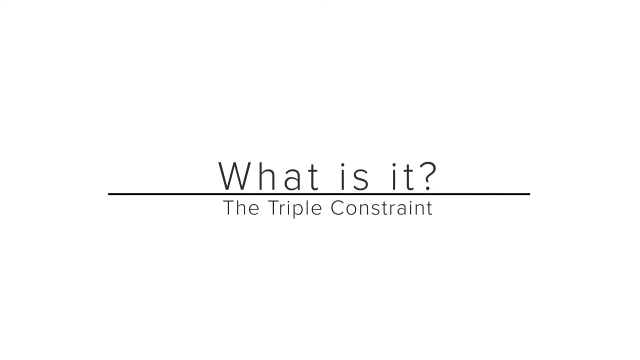 basics. what is this? why is this important? and talk a little bit- just a little bit, i'm gonna try- about some of the use cases and, um how you might leverage this tool. let's start with the basics. what is the triple constraint? the most basic definition? you can just google this and find it. 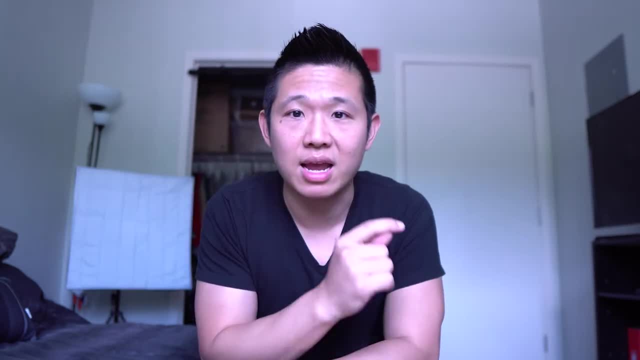 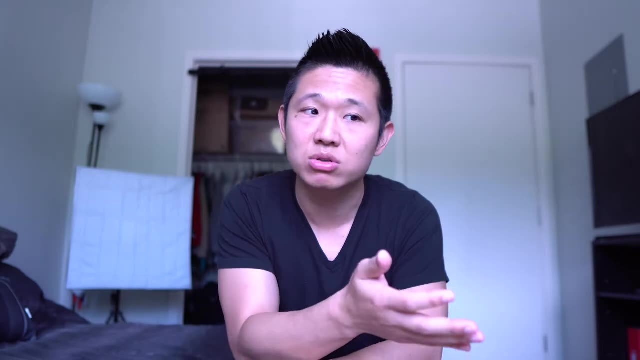 it is the three most significant restrictions on any given project. and when i say this, it's not just pharmacy informatics, it's any project out there. you could be a pharmacy student working on a project, pharmacy resident working on a project, a medical student working on a project. 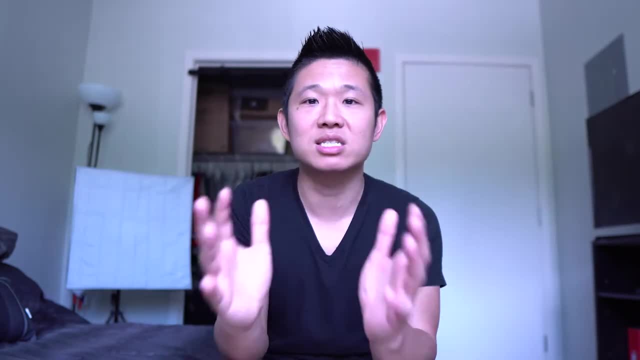 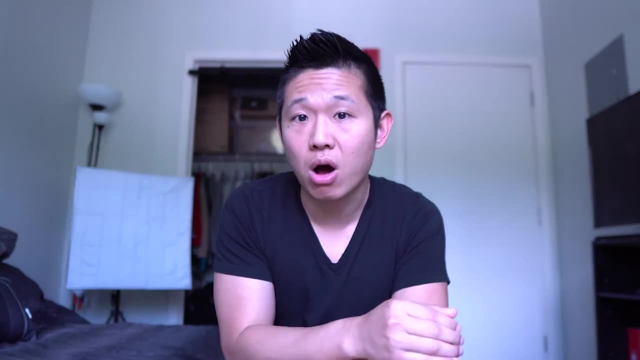 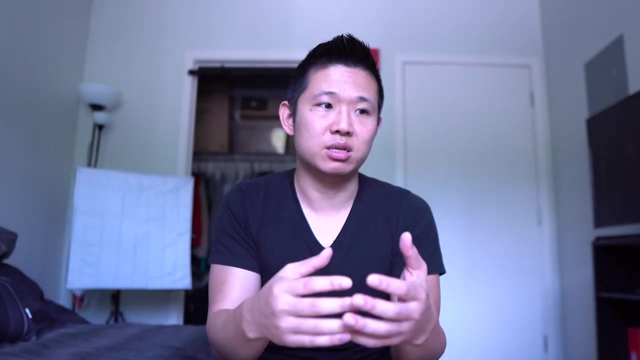 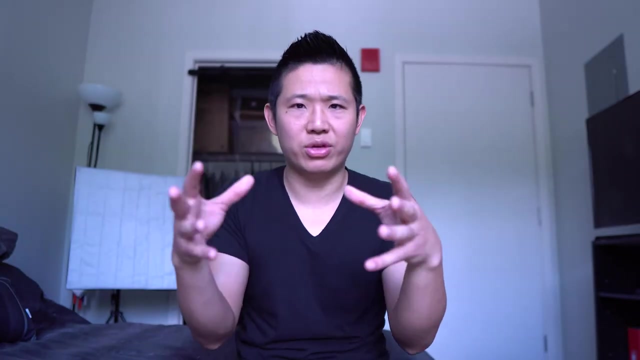 uh, a undergrad doing some homework assignment, working on a project doesn't matter any given project. these are the three most significant restraints or restrictions, and the three are scope, schedule and time. other names for this is the project management triangle or the iron triangle. i like the triple constraint. it sounds cool. there are many other things you can. 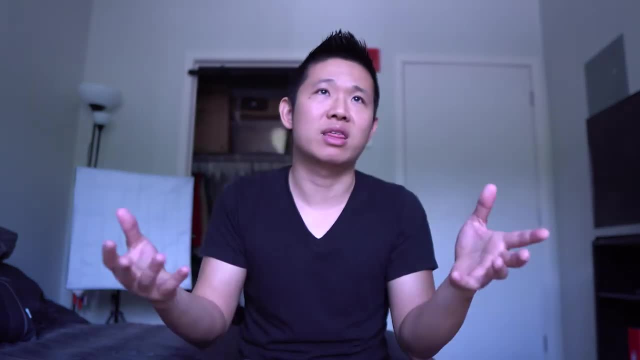 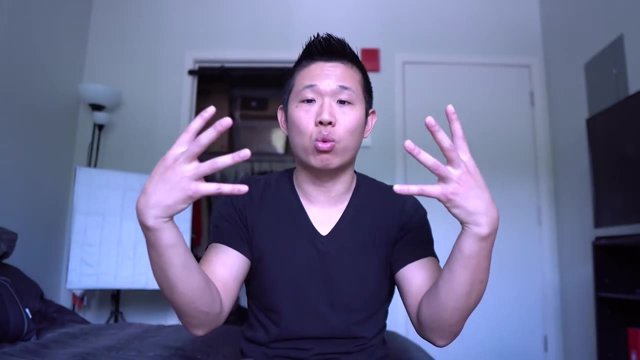 talk about with, just like basic definition. uh, something i think would be important to highlight is: within the triangle, usually quality is in the center of it. so these three things- how well they work together or how well they're defined, or how well you achieve the three things, 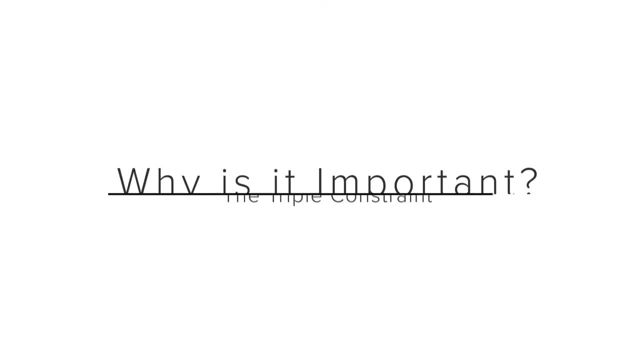 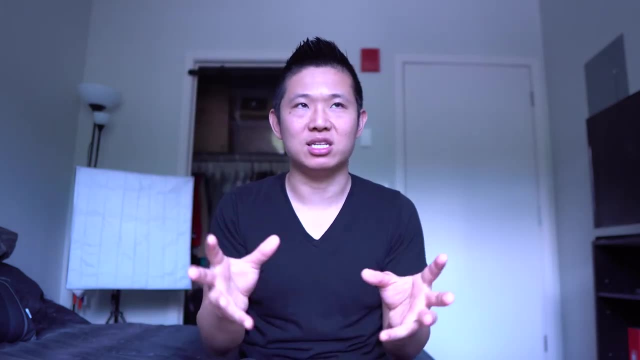 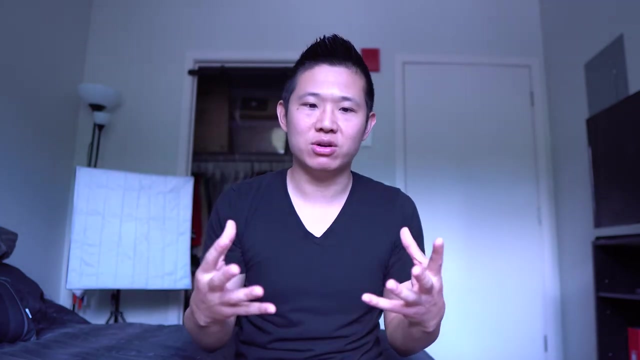 you will get quality in the middle. so why is this important? and basically it comes down to the the fact that these three things are all kind of interconnected. you can't really change one of them without really impacting the other two, and the translation here is basically that. 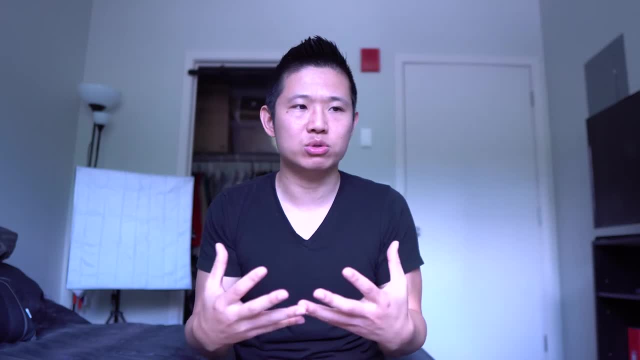 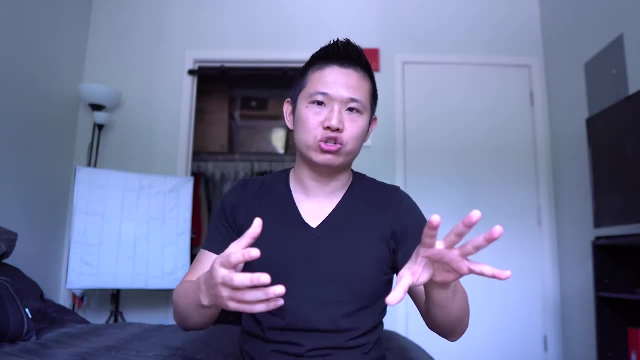 you can't have it all in a sense, and most examples will kind of talk about the pick two idea, where when you can only have two of them, if you constrain one of them. and so let's, let's use an example here. let's say you have a project. 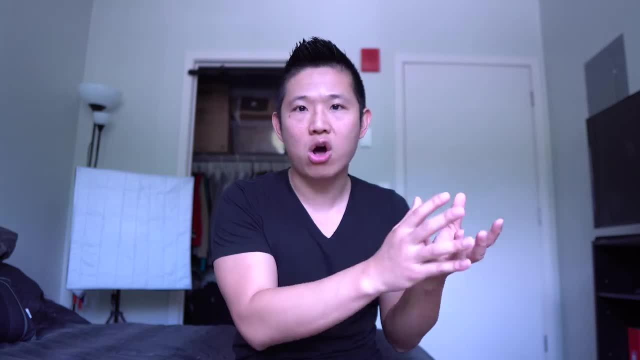 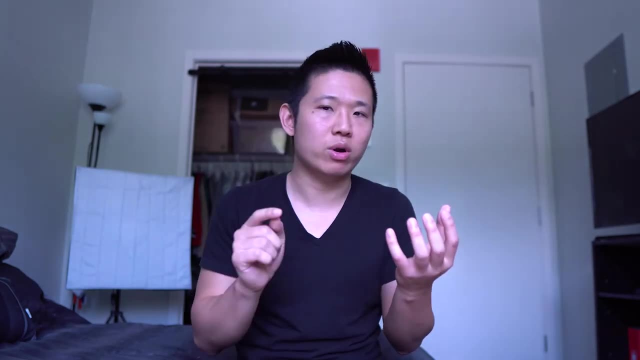 that has very tight resources and your costs and resources are constrained. then what may happen there? because you're tight in one area, you can only pick one other one, so you might end up having a lower quality project or a project that may be in the center of a project or a project that's. 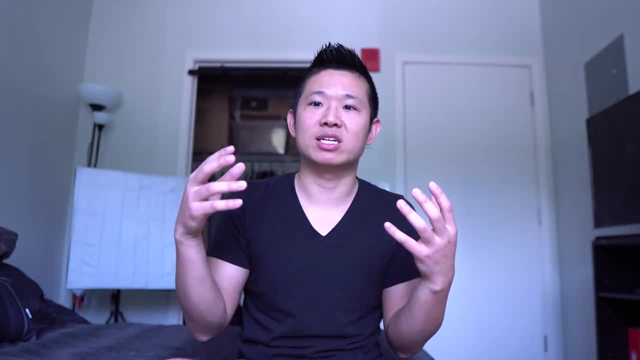 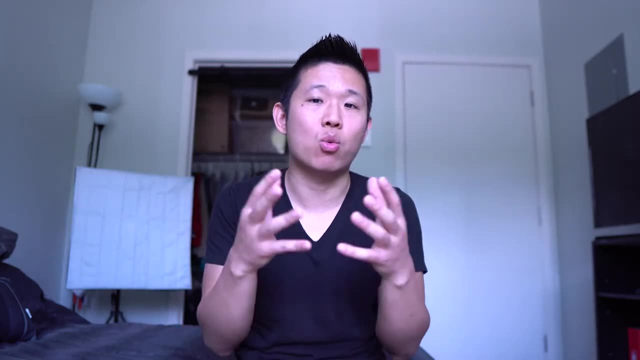 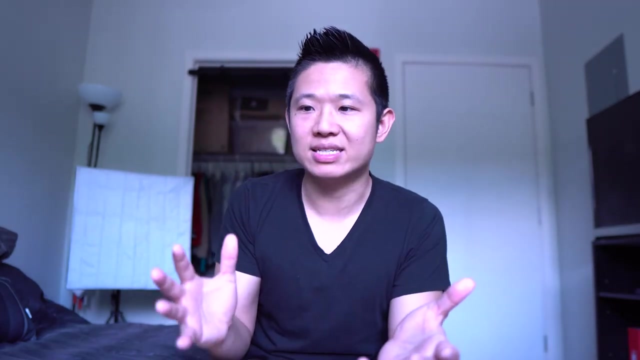 take a longer amount of time, or a project that has less functionality or less features, because your scope needs to be decreased. so that's kind of the translation of why this is important, and I think I want to highlight this because you know, as someone who works in informatics, this kind of triangle. if you 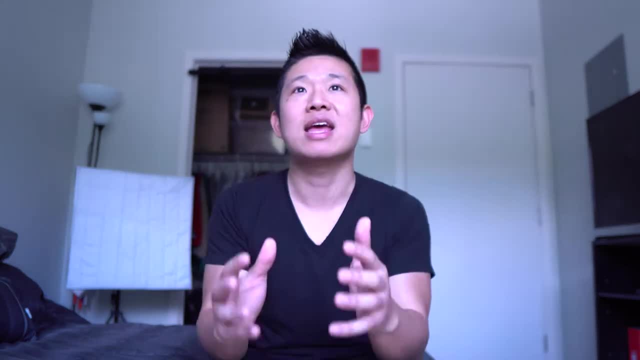 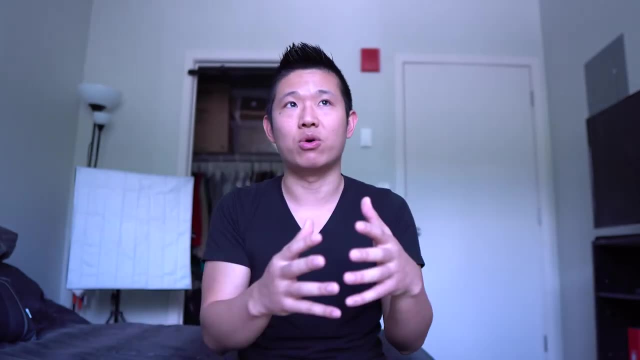 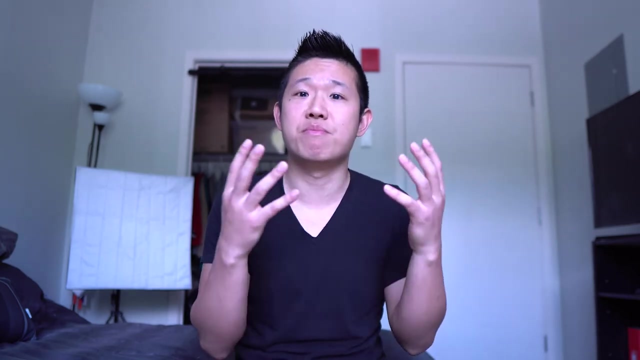 will, is what you base a lot of your decisions on and how you want to convey, convey your messages to various stakeholders. for example, you, you have a project and typically that's just a simple example. you usually have many, many, many projects that you might be balancing at any given time and you have 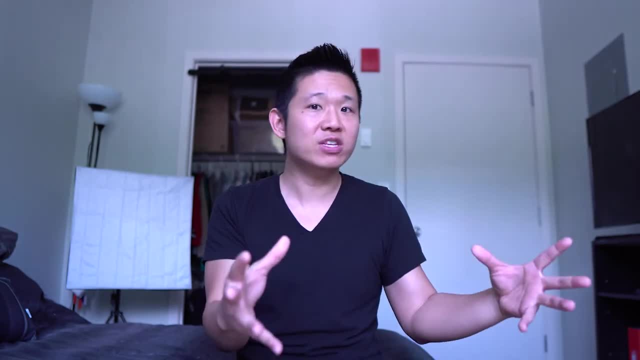 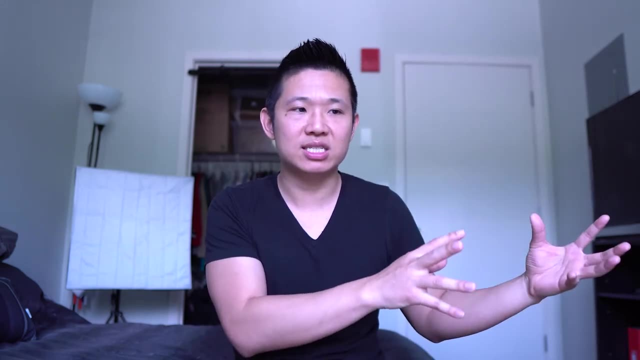 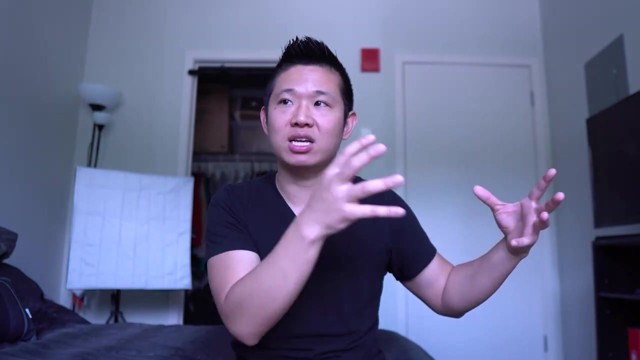 to have conversations with them. because, let's say, you have 15 projects that you are working on or actively involved when, at a given time, and five of those projects, their stakeholders want to increase the scope or speed up the project. well, you can't without impacting other things, so let's. 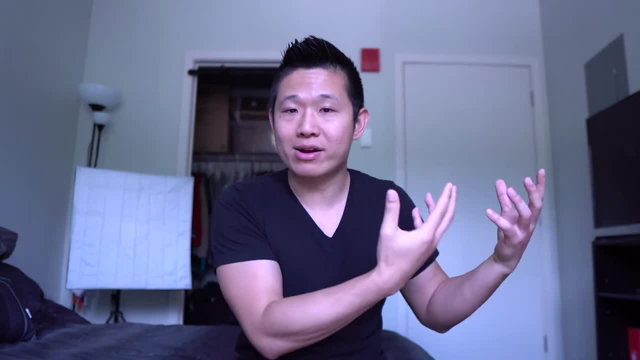 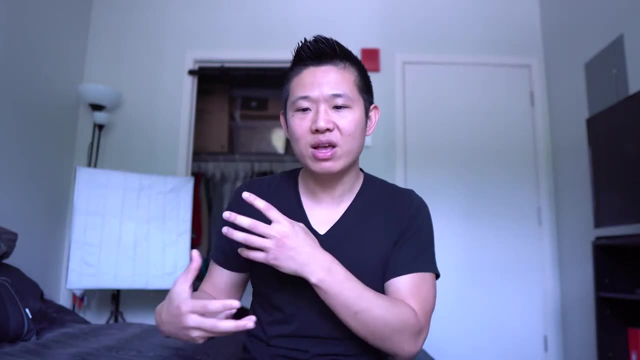 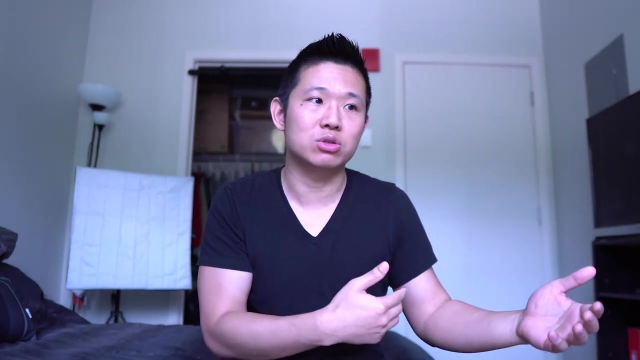 say they want to speed up these five things. well, it requires more resources, and where is that resource is going to come? it's going to come from the time you're spending on other projects, so you have to have conversations in which you can ask them. you know, is this important? what is the the reason why we need to do? 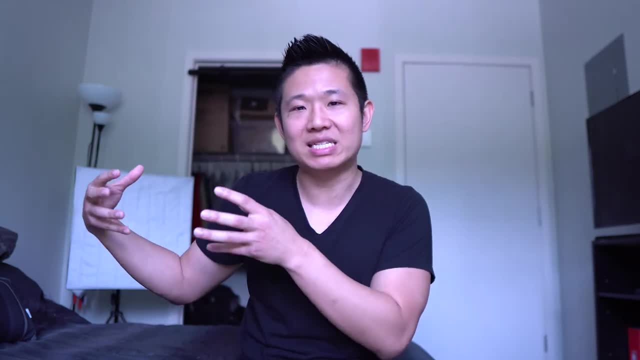 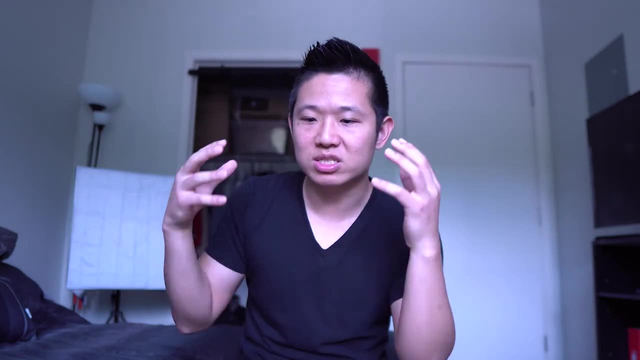 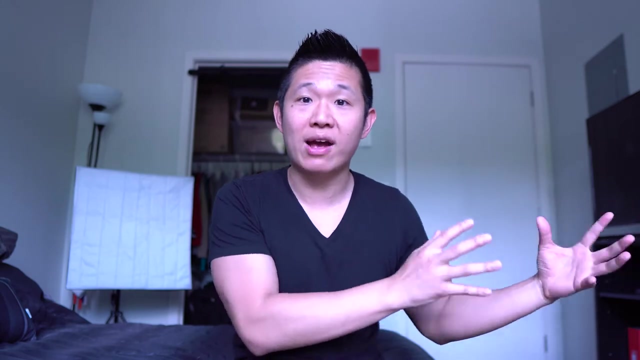 this because other projects will be basically deprioritized in that sense, but it's, you know, it's okay. the thing is why it's important is you, as the person who are part is part of that project, need to take that into consideration in order to drive those conversations. you you can tell them like: is this okay to? 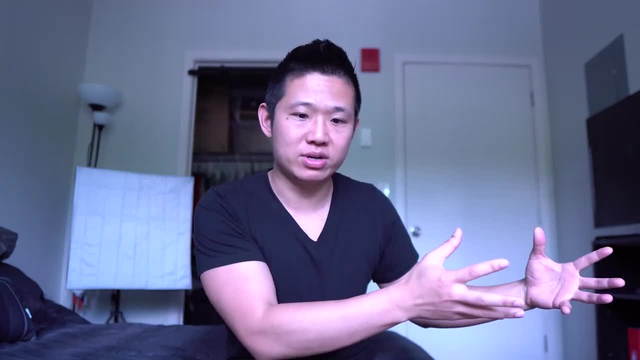 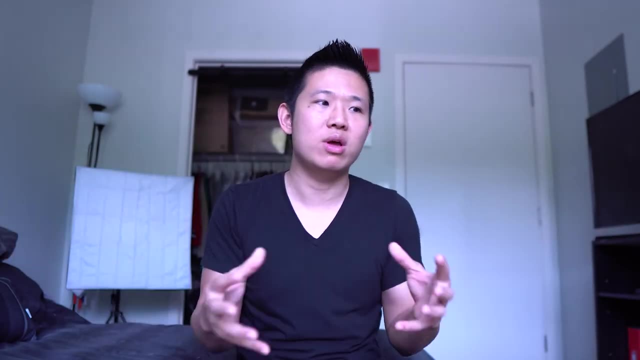 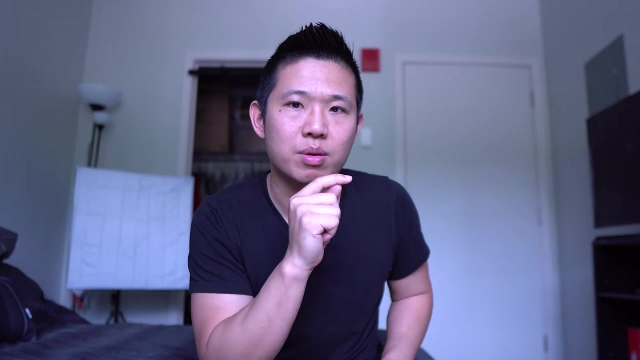 deprioritize. you know, or should this not be prioritizing? the basic idea is that you have to make decisions and think about everything as a whole you can, how you convey and talk to your stakeholders- needs to have all this in place, and I'll talk about this a little bit more when we talk about some. 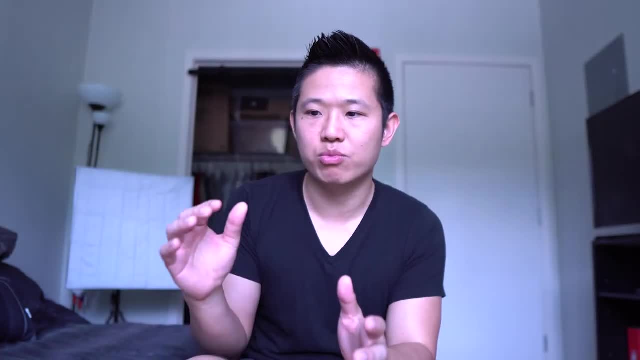 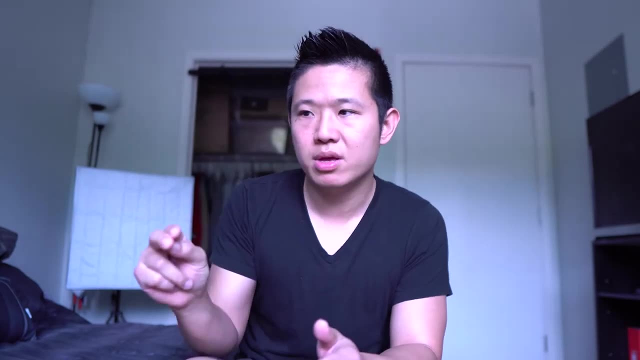 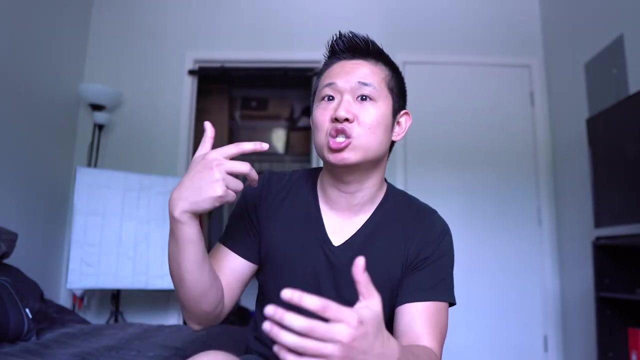 examples. let's let's talk a little bit more concrete here and move on to talking about a little bit more about each one of those three things, starting with scope. so what is kind of scope? it's more of the nuts and bolts of the project. if you will, it is the specs, or the build specs of that project. so let's. 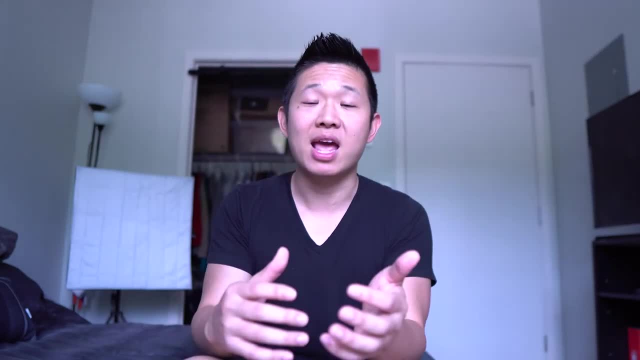 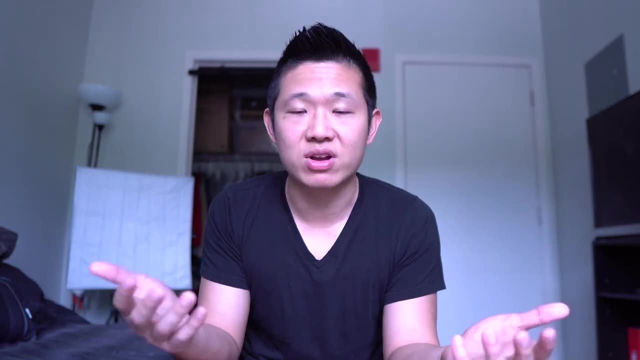 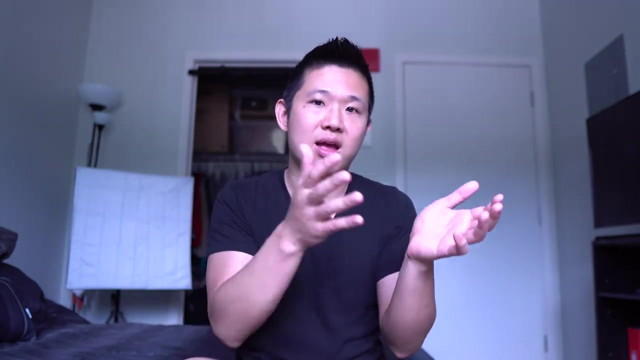 use an example. let's say your organization wants to develop a pharmacokinetics calculator. to develop a pharmacokinetics calculator. to develop a pharmacokinetics calculator for your pharmacist to monitor drugs that have a narrow therapeutic index and maybe help them calculate what an appropriate loading and maintenance dose may be, and even help them recalculate it as they 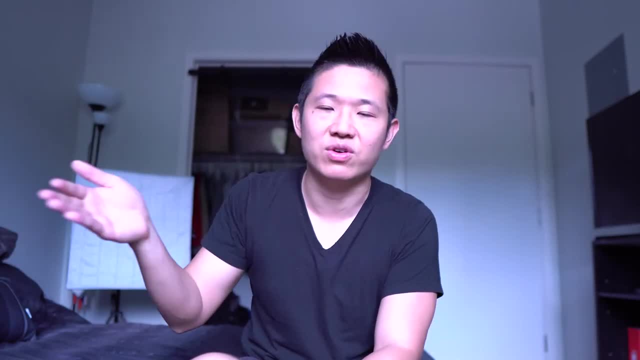 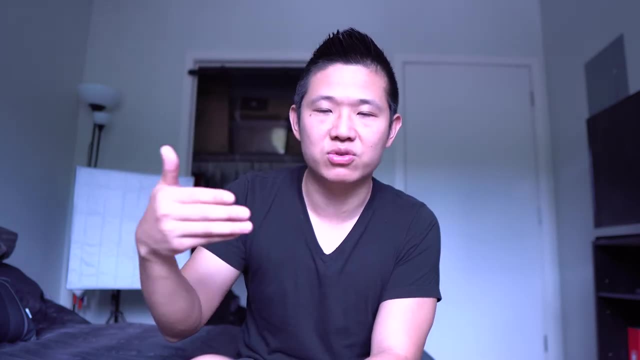 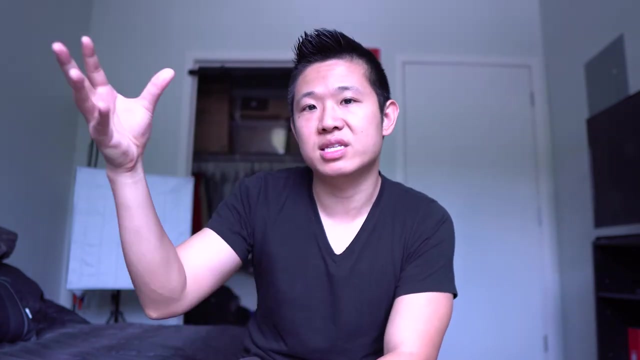 progress through the day, so as the patient changes, the renal function changes or kidney function changes, whatever may be, when those things occur, this will help them make appropriate decisions. for pharmacokinetics scope, you have to define clearly what drugs meet this definition, what drugs should be. included in the project? Should it be all drugs that have an error therapeutic index? Maybe there is a patient issue, or patient safety issue, I mean, or a joint commission requirement where certain drugs are more prone to error and you want to target those drugs. 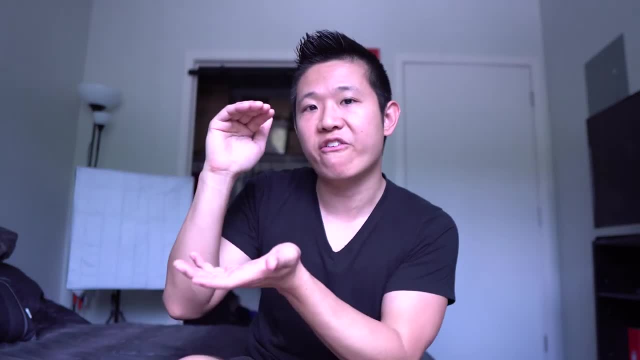 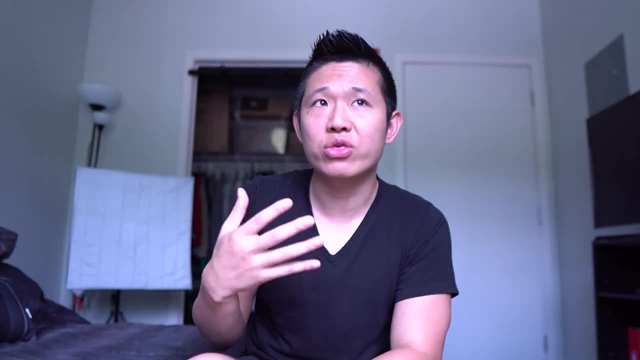 for inclusion in the project. So you need to clearly define all of that to determine your scope. And something else with scope is complexity Within informatics. it's a field and I shouldn't just say informatics, it's just in projects. 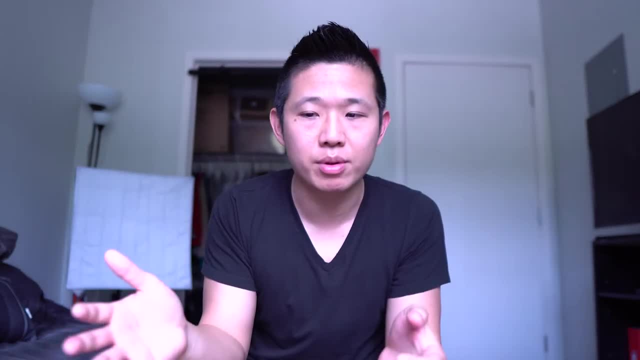 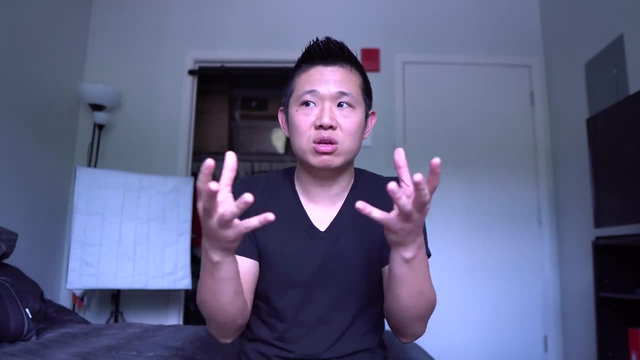 in general, there's usually more than one answer to any given problem And depending on the solution that you choose. so for this pharmacokinetics calculator you can do it, let's say, three different ways. You can have a student on rotations. create an Excel sheet. 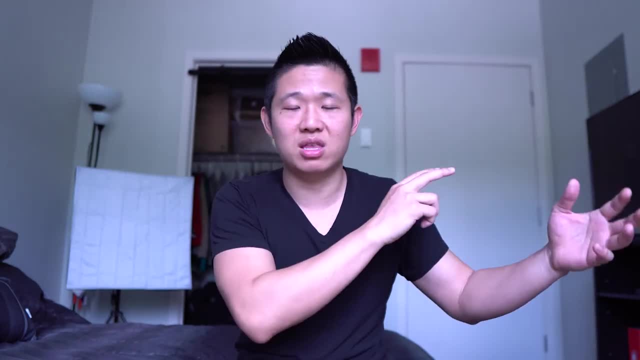 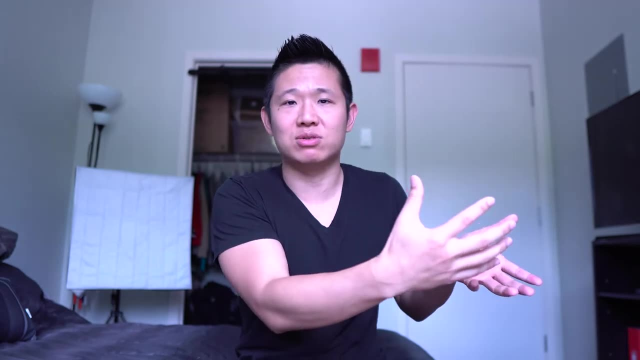 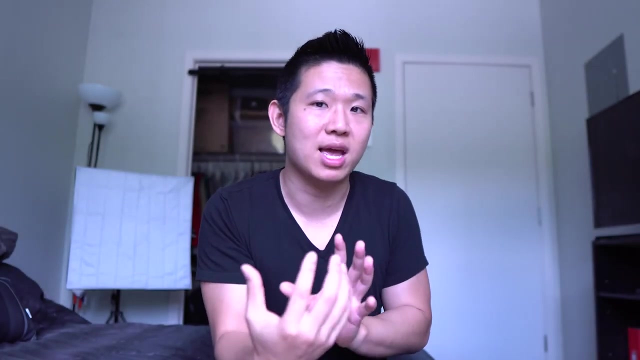 For every single drug that has the pharmacist input, the different parameters that will drive the loading or maintenance dose of a given drug. Pretty basic. You can probably have a student project do that and that's not that difficult of a scope. But let's say you want to make it more complex and make it integrated into your EHR. 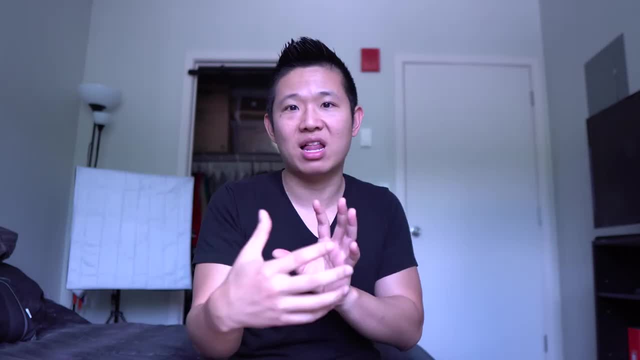 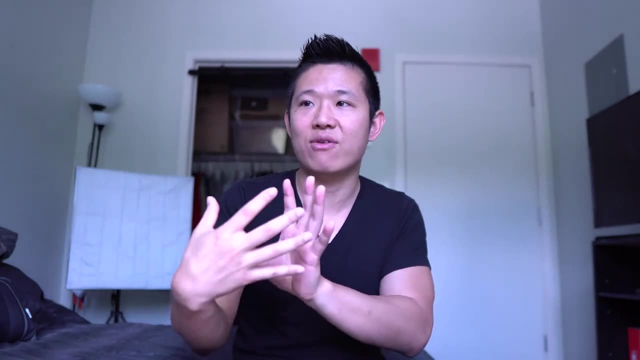 Let's say, for example, your pharmacist has this drug like mancomycin, and you want them to use this calculator. you want to integrate it, so you provide a link every time that drug is ordered To this Excel that the student programs. 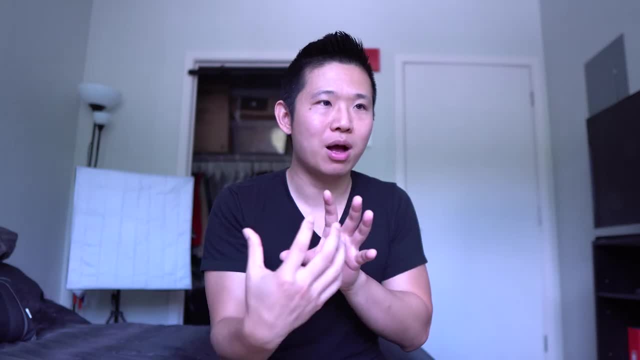 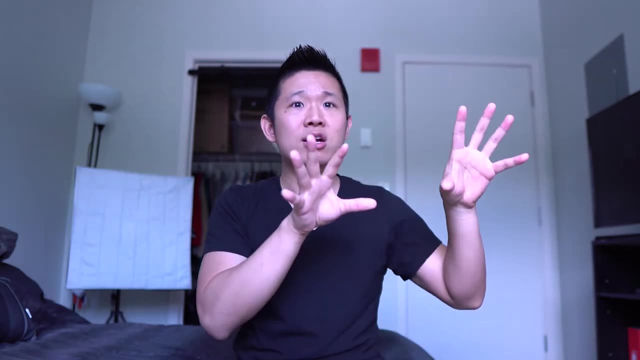 That's an increase in scope, but it's probably not super complex because you're just linking to something else that's outside of the EHR, But technically it's within because there's a link there, you know. So that's two different ones. 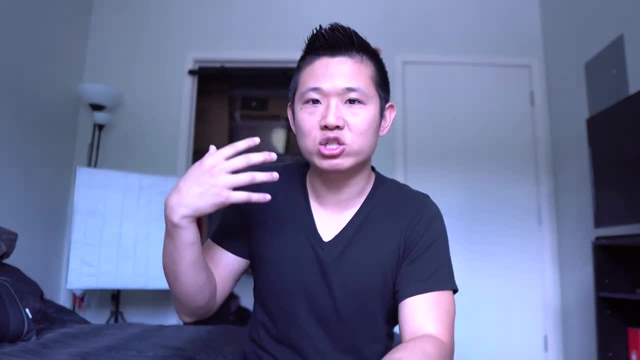 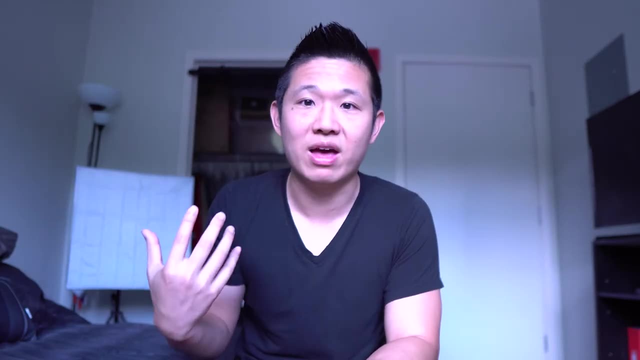 But then you can go a level further and say: well, I want it to be integrated into the EHR, I don't want my pharmacist to input anything, I want the EHR to do all of that for me, And so they would look up the patient's weight. 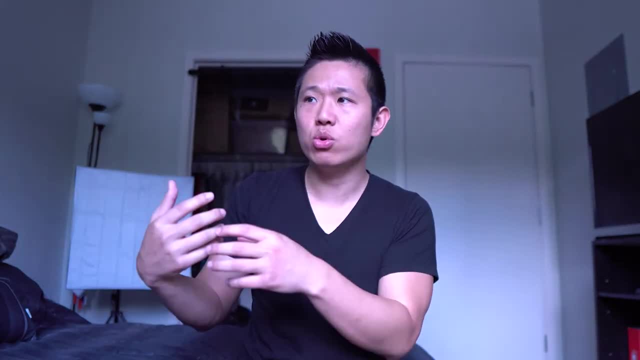 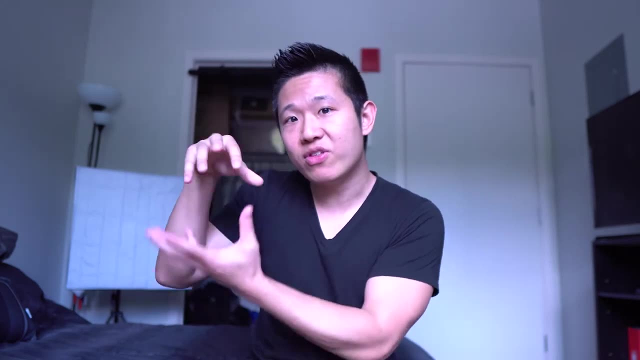 They will look up their. They would calculate the very specific makes per kick dosing for a specific drug based on what's ordered. all of that inside the EHR. That's a whole nother level of complexity and you can. you might need to involve multiple. 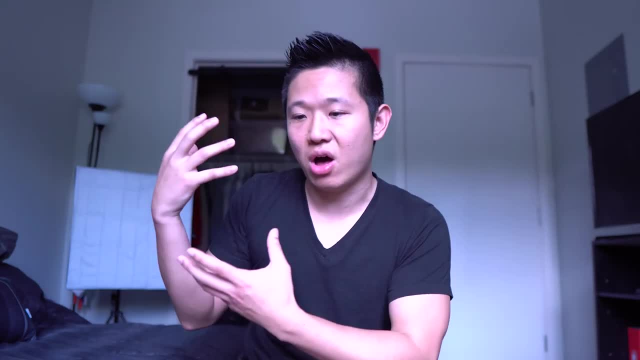 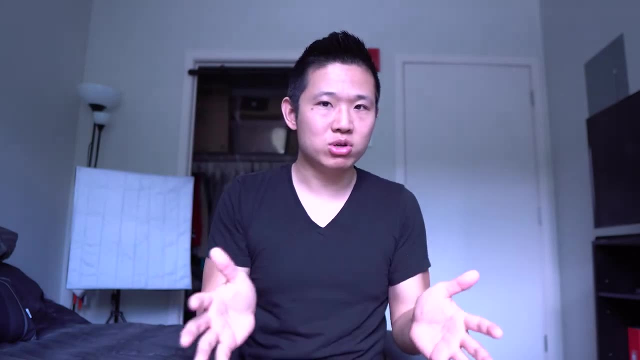 teams, where you probably need to involve multiple teams, but there's a lot of other complexity, complex things that need to be considered when doing these types of things. So that is what I'm talking about with scope. There's different things And most of the time these questions can't be answered without talking about the other. 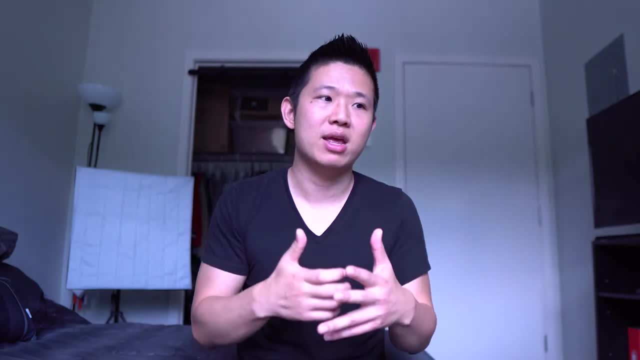 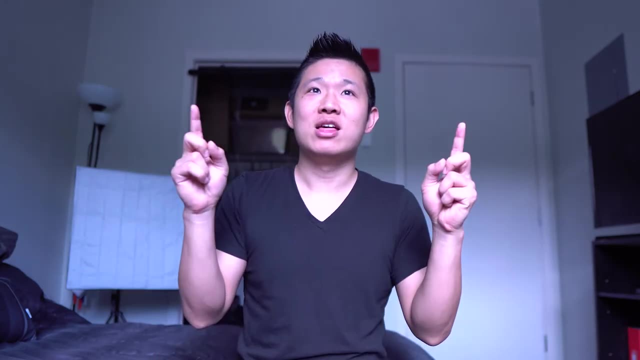 things, How much resources do we have, How much time do we have to implement? So all of these things need to be considered, And I probably spent way too much time talking about this one thing, So let's move on to the next. 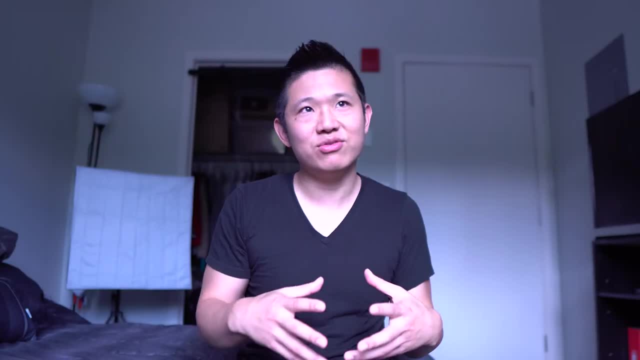 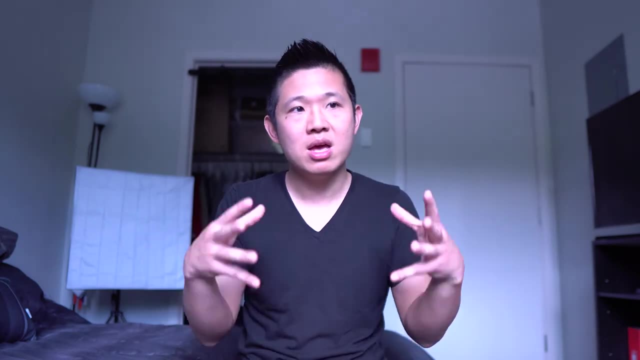 The next thing is resources, And for this it's kind of common sense. Actually, this entire conversation and video is probably common sense, but probably people don't think about it all the time. resources: you know how much do things cost, How many resources? 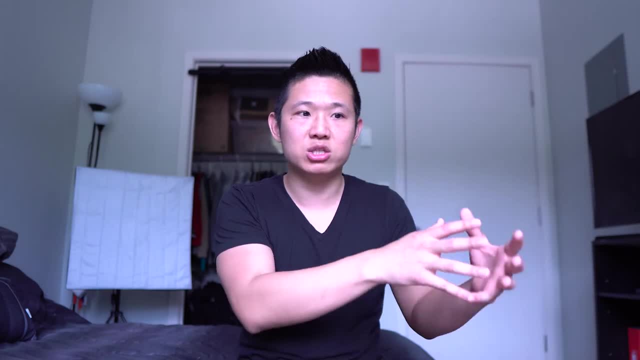 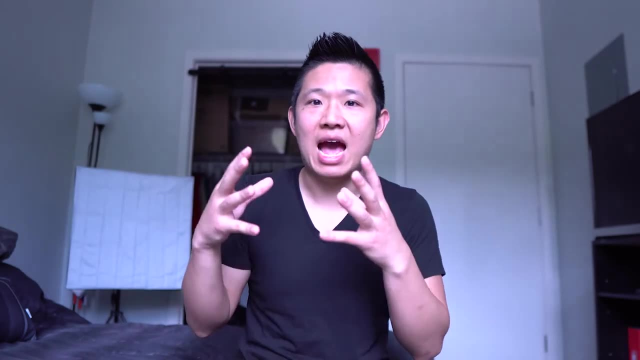 Do we need? Do we need one analyst devoted to this project? Do we need two analysts? Do we need multiple analysts? Do we need a dedicated project manager? And it's something else that I think a lot of people think about is how much time do. 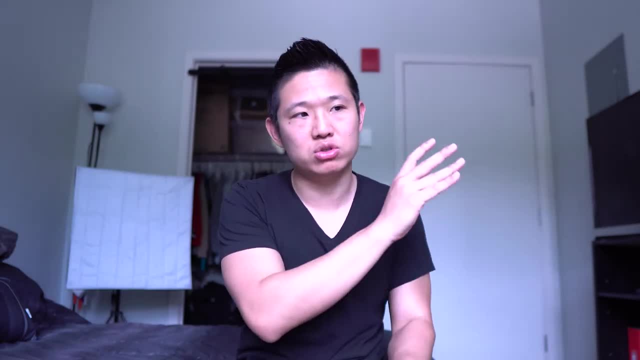 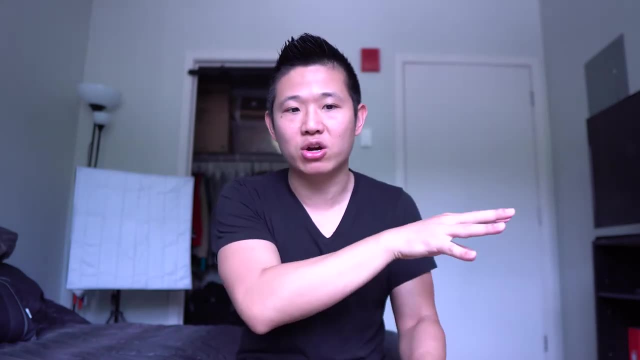 we need to take away from your stakeholders, your end users, your subject matter experts or your SMEs. You know you need to bring in a physician or a pharmacist or a nurse or a administrator. You're taking time away from them when they could be doing other things. 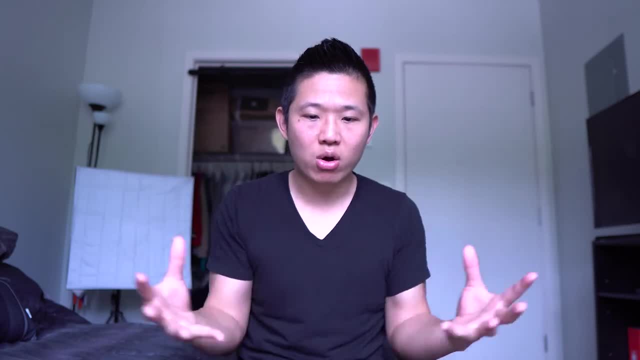 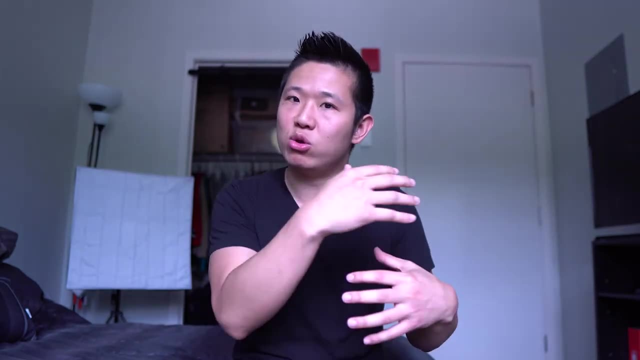 And that has a cost associated with it, Right, So that all factors into the cost and many projects usually is constrained by a budget, So there's only so much leeway you have in this area, So that needs to be considered. Now let's move on to the last one, which is time. 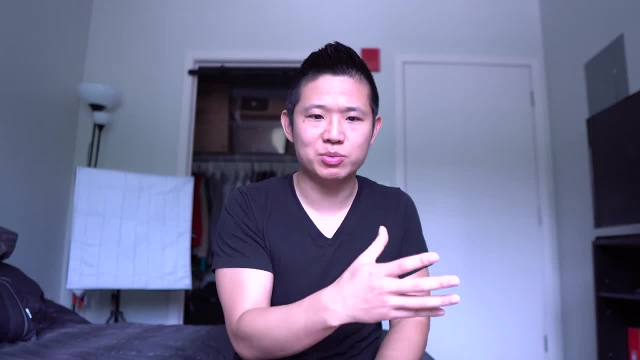 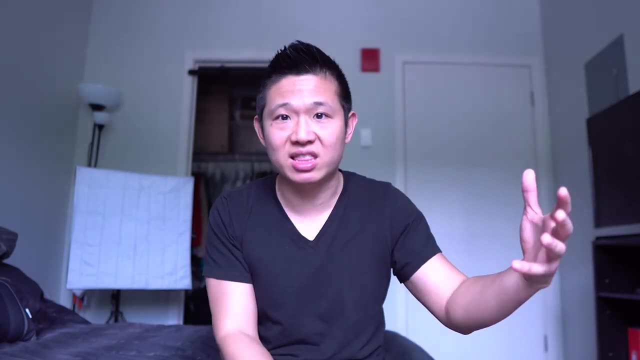 And this is pretty self explanatory as well. It's just basically: when does your project need to be completed by? and many things can drive this decision. You know you have your basic things of what is required in a hospital accreditation or something within your policy. 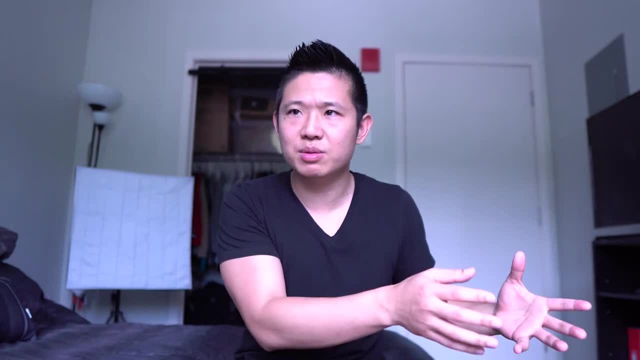 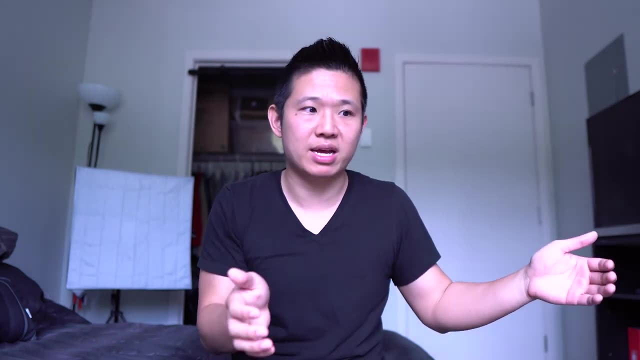 Yeah, You have policies that require something to be done by a certain time. Those are pretty simple, You know. just need to have something done. Here's the deadline. This is how much time we have to do this project. But there are other things, like maybe a new building is in place. 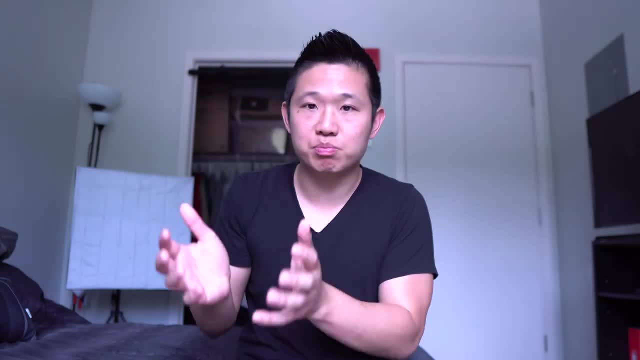 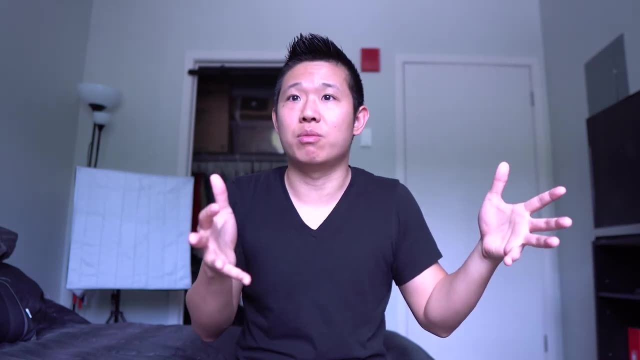 We want to get things built before this project, or I mean, this building is complete. So you have this certain allocated time to complete a project, or you might have, you know, some emergent thing where a patient was harmed or some safety issue that just 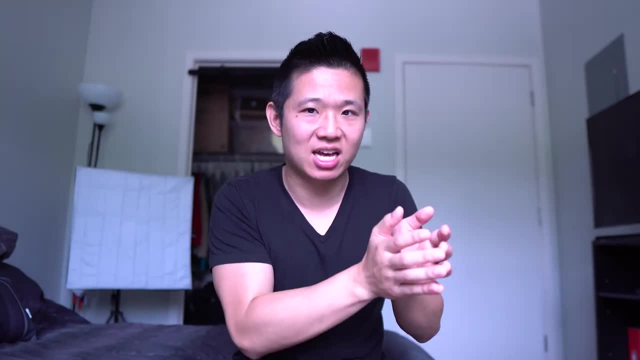 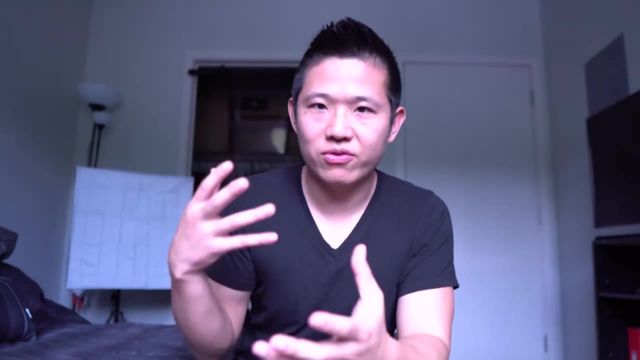 needs to be addressed in a very short period of time, Because we need to act on this and take care of it. So you have this constrained time, So all of that kind of drives the timelines, Kind of wrapping all of this up as an informatics pharmacist or as anyone who practices within, 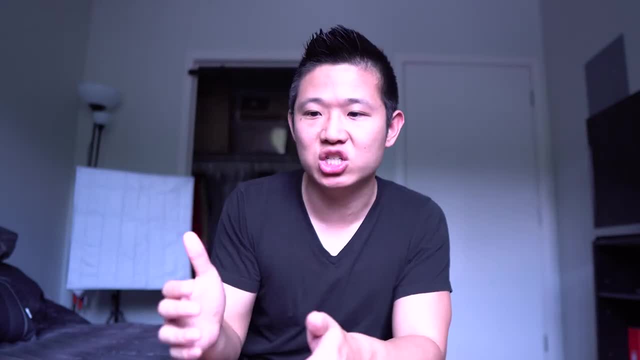 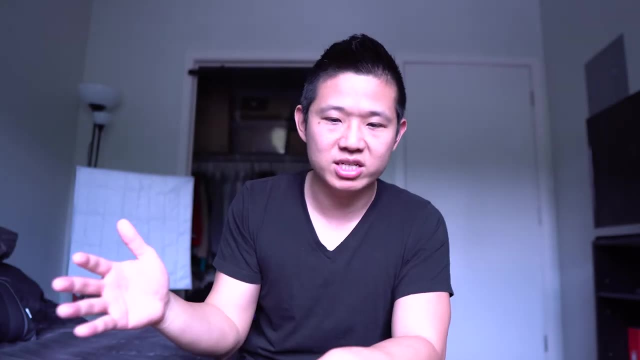 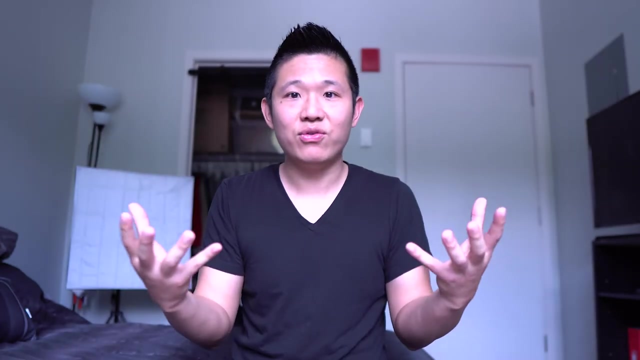 the field of informatics. you make these kinds of decisions and these three things should be on your mind on a day to day basis, Because as you work on these projects, your stakeholders undoubtedly will want to make changes, Especially in your in life. things change. You know whether it's the deadline gets shortened or the deadline gets longer. you don't usually see that. I mean it depends on the project. Everything's very it depends. So then you have like scope. you know there's new features that come out, there's new functionality. 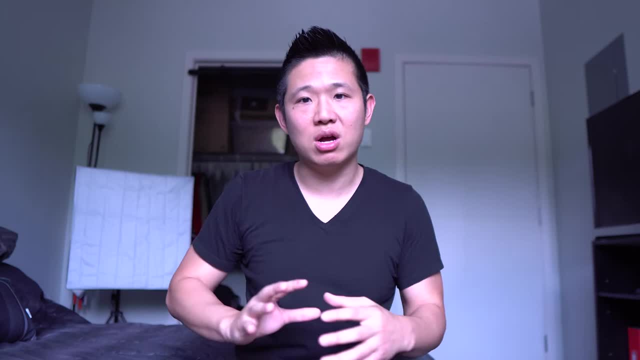 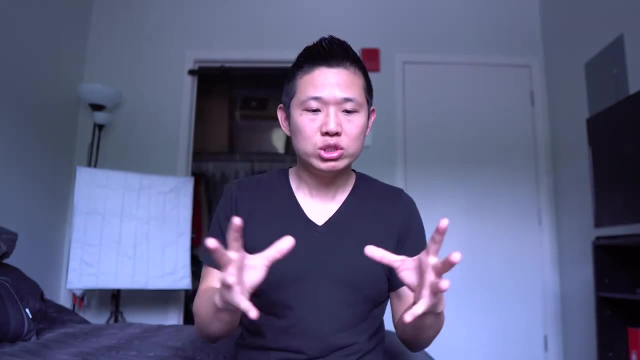 but when you increase scope, you know it has to come from somewhere else. Whether you have to hire more people or you have to take longer to complete a project, you know it depends. Those three things you. I can't harp enough. 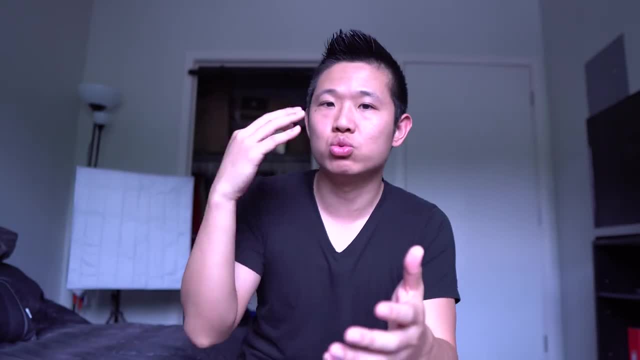 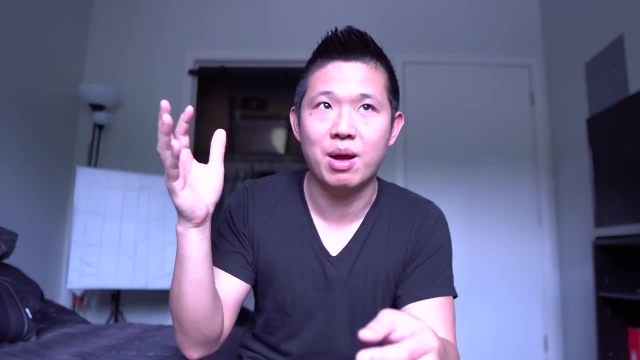 You have to think about those things. So it's really important to have this on your back of your mind And, more importantly, when you talk with your stakeholders and I keep talking about- I'm probably repeating myself, but these kinds of things in the back of your mind should. 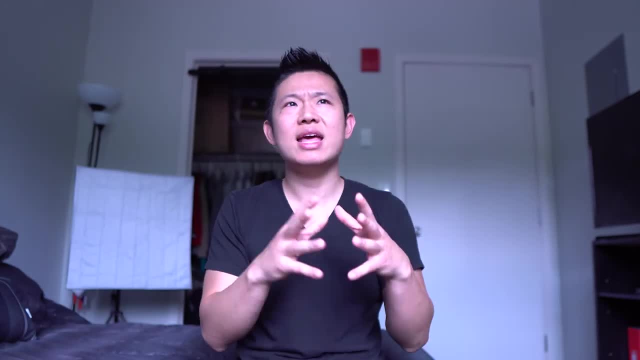 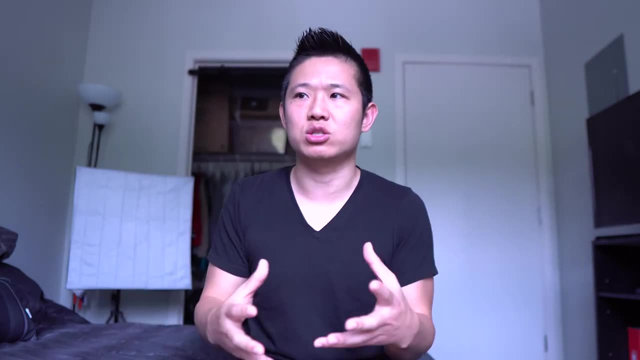 be driving the types of discussions you have with your stakeholders, And there are. it's not that it's a bad thing, you know. it's just something that helps you develop those contingency plans When either your scope needs to be increased or you get a shortened length of time, or you. 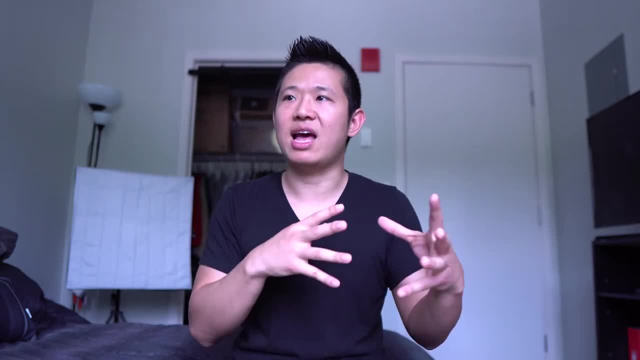 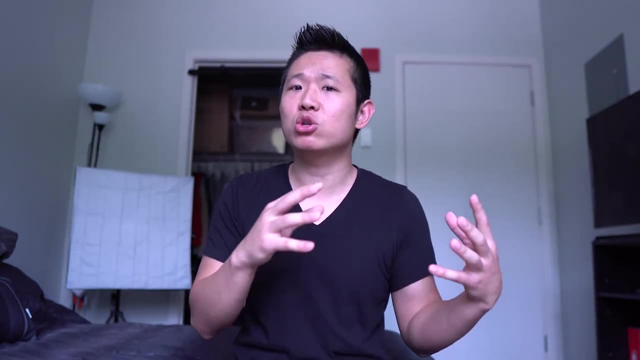 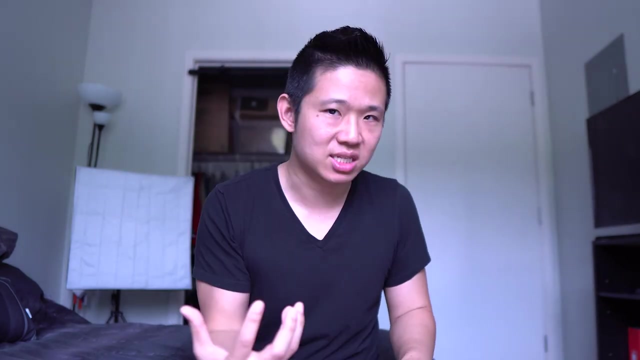 have less resources because maybe someone quit- things like that. When you have these kinds of things within a project- and of course your project will have those things- then you need to start thinking about what do I need to do? What do I need to move or what do I need to impact to make sure my project succeeds? 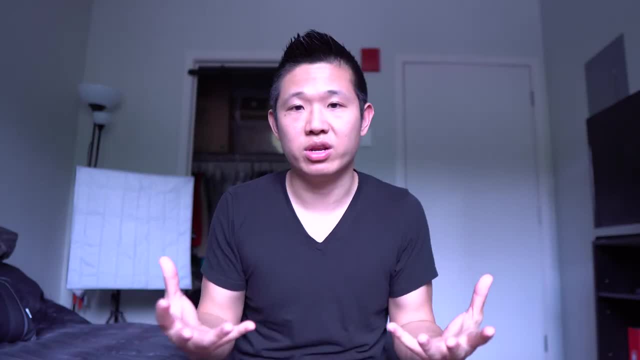 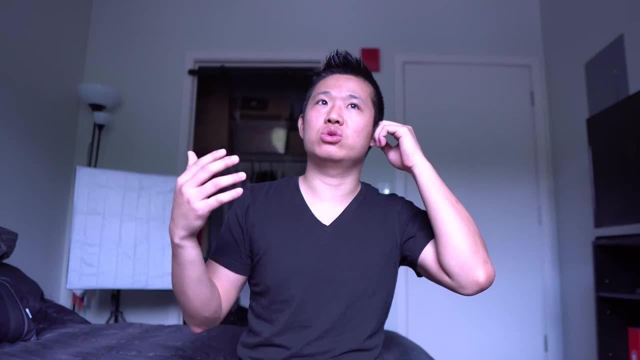 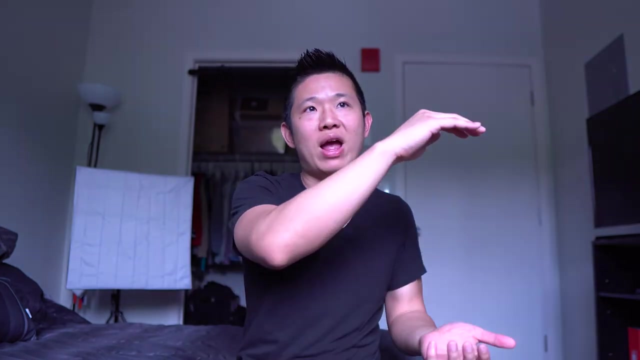 And there are many things you can do when something changes within a project, because there's always something that will change, Yeah. So let's use a quick example. Let's say you know you need to do something extra. Let's say there's a new accreditation requirement that requires you to further add. 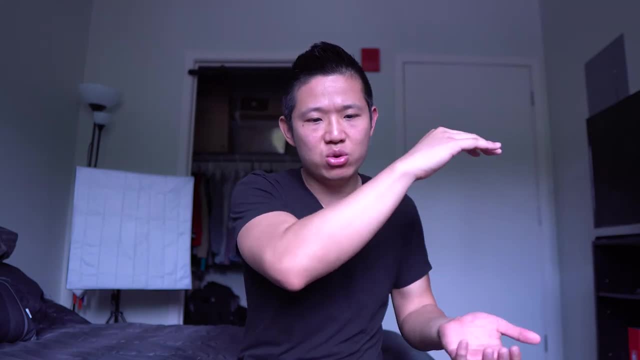 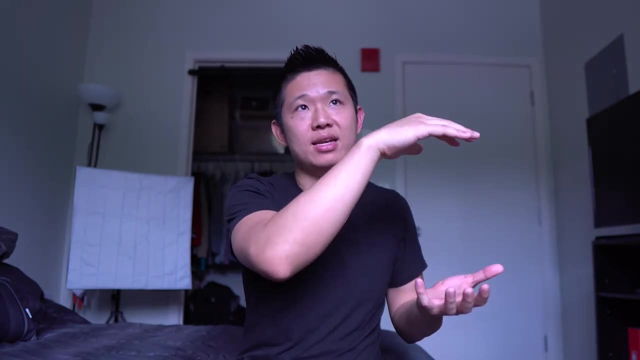 Let's use the same example: pharmacokinetics calculator. Let's say: you need to do a better job of monitoring digoxin and you want to develop a calculator for that, And that's increased scope if it wasn't already included in your project specs in the beginning. 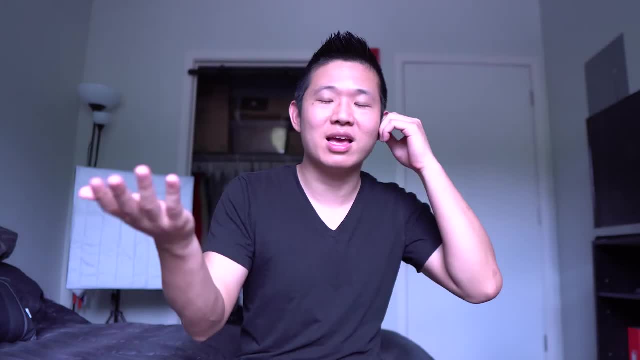 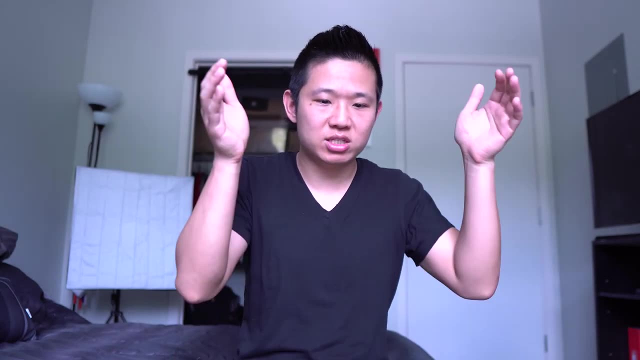 So now you have an increase in scope. It's kind of probably small scope, but again it depends on the complexity of the project, but you do have an increase in scope. So now what are you going to do? Let's say the timeline can't change, because this you have to deliver it by this accreditation. 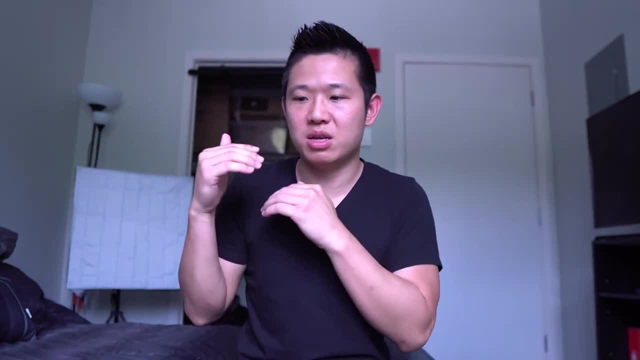 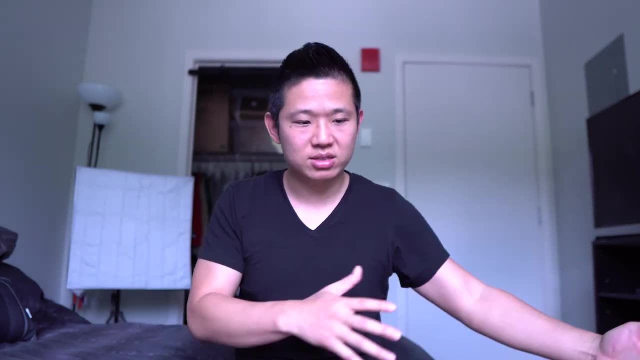 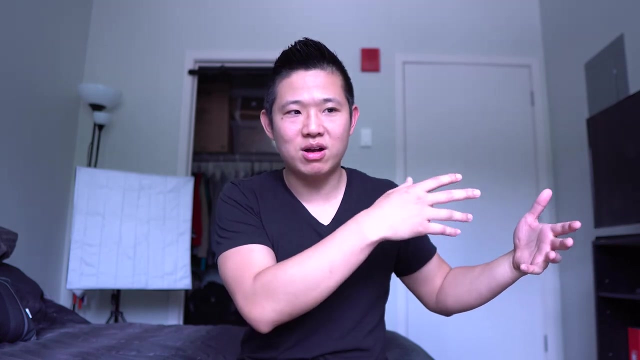 guideline, and now you have an increased scope. So the only thing you can change are your resources. So how do you change your resources? And there are a variety of ways that you can do this. Obvious answer is: you can hire someone well. even with that said, there's more complex. 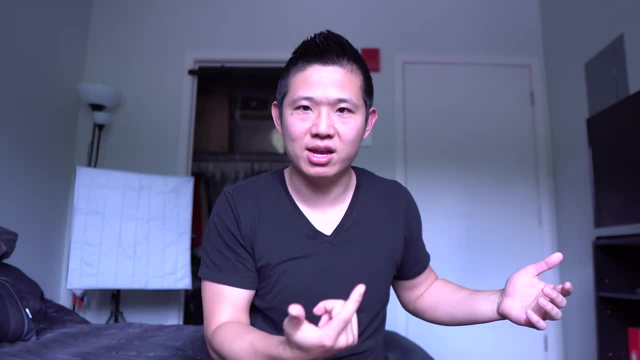 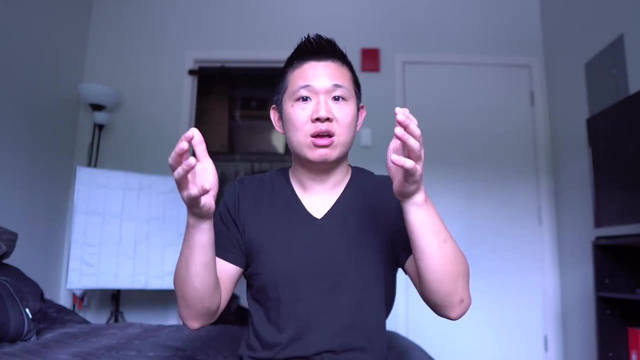 things to consider: that when you hire someone doesn't mean you're automatically increasing resources. Well, that person needs to be trained and you're going to take away time from individuals that are on the project, which will make them less efficient to train someone else. 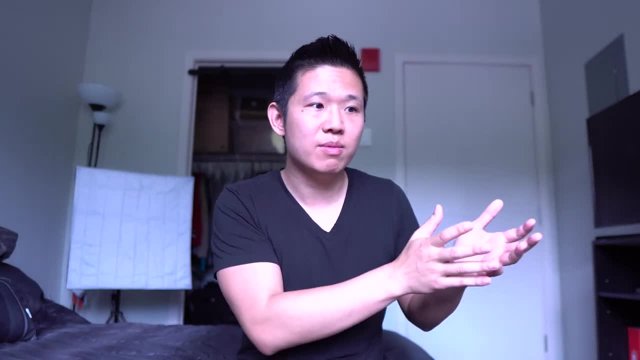 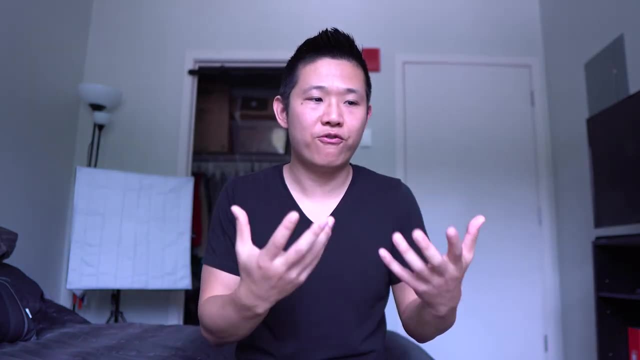 So hiring someone isn't always the answer. It could be if we're thinking about maybe something longterm. you can train them over time, and over time you're going to have another resource that can help further that project along. But that's one thing you can do. 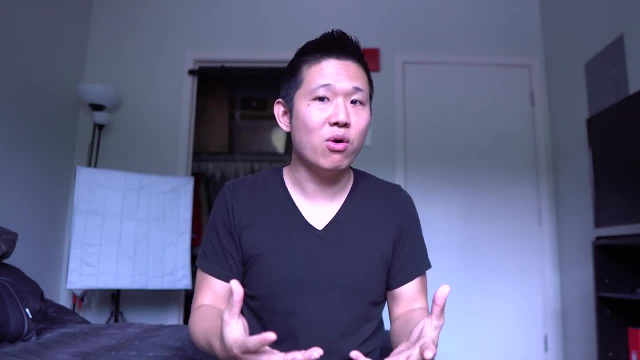 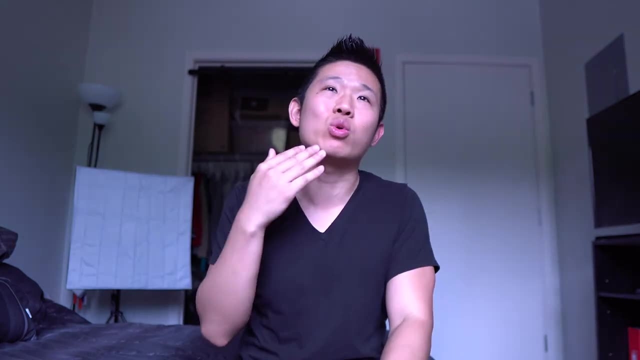 Another thing you can do is you can have your workers Put in some overtime. Now that usually is a temporary solution, but it's a workable solution. Maybe it's like there's something that just quickly came out of the woodworks and you 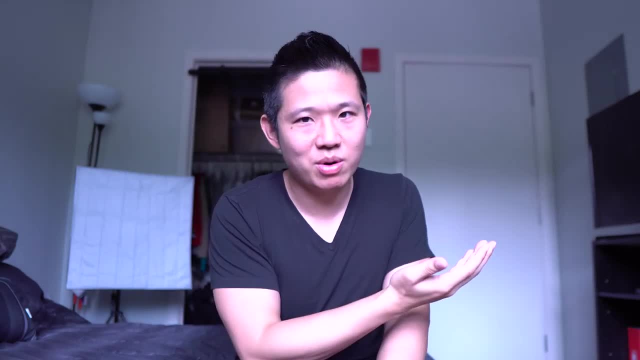 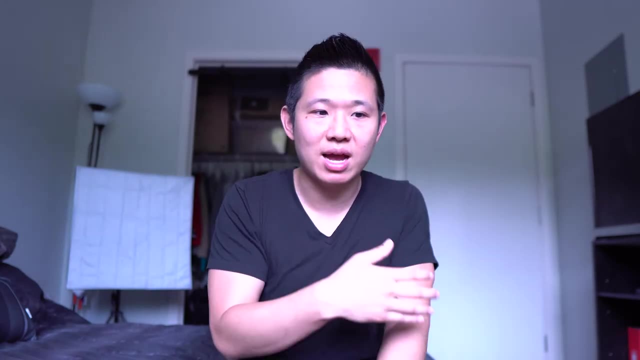 need something completed by tomorrow. You obviously can't hire someone tomorrow, or maybe you can, but you know it's very difficult and you know you ask your workers if they can put in a little bit more overtime to get this done and accomplished by the very next day. 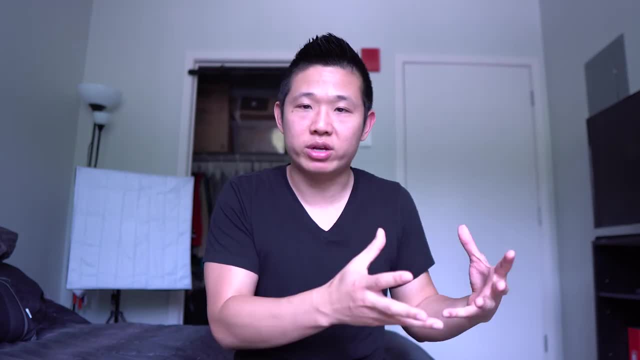 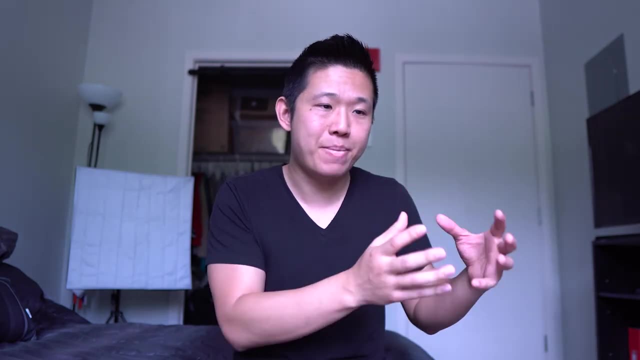 That's something to do, but you obviously have other things to consider, like working and burning people out. So you have to be careful with that as well, because the last thing you want to do is you have your best workers quit on you because you just made them work for like three months. 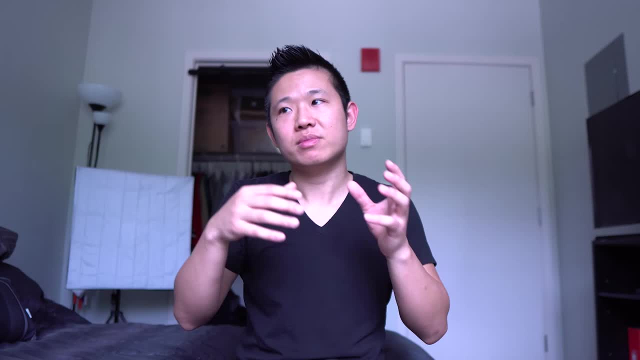 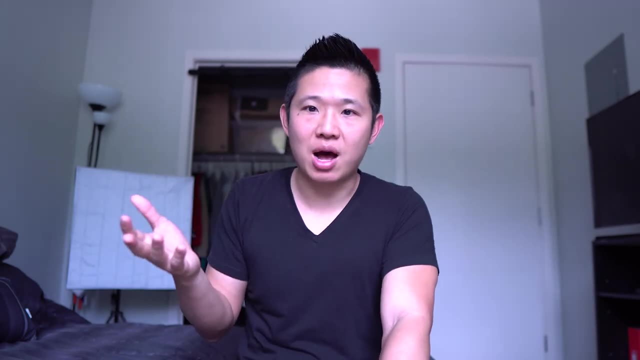 straight. That's not cool. So something else to consider- And the third thing is something you can do which is kind of creative, in my opinion- is you can shift resources, and this is probably a common strategy. about a lot of supervisors and managers do is where you don't have the resources. 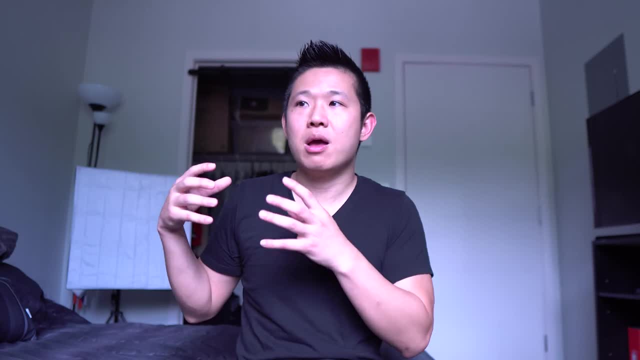 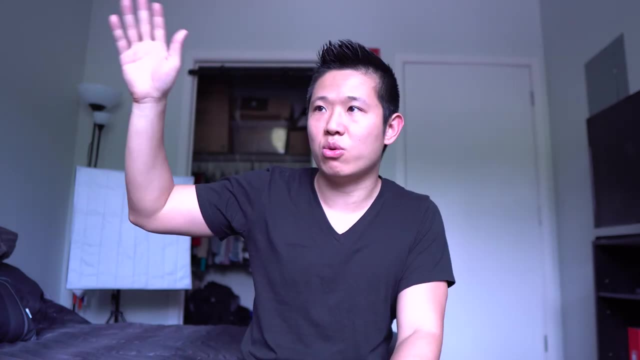 You can't hire someone in time. You don't want to burn out your workers. But you can look at different resources, maybe on different teams or within teams. Let's say: you know this team is doing excellent, You talk with them. 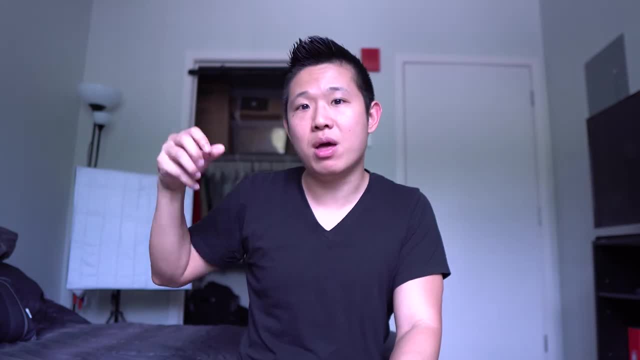 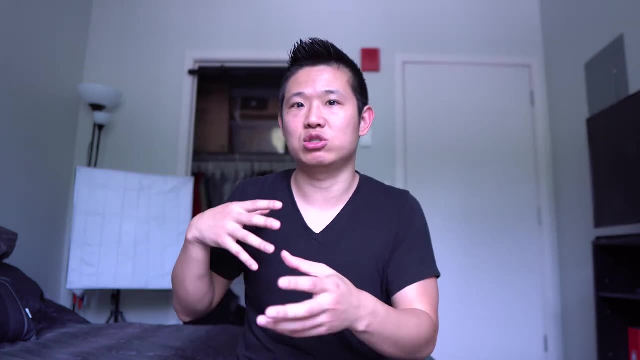 Maybe you can bring them over for a short period of time or permanently and have them help with your project or you- you know someone has experience in this and you can pull them temporarily to help with that. So kind of shifting resources. you're not hiring anyone. 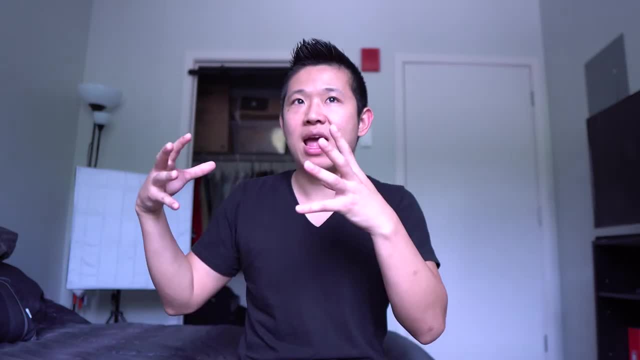 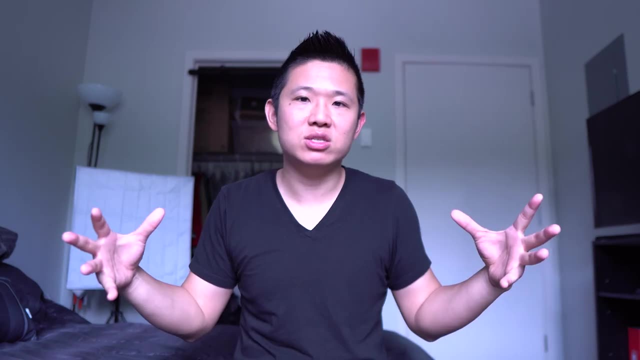 Your resource cost remains the same in a sense, and you can still get the project and meet those project deadlines and meet that new project Scope. So those are all things you can do and that's that's what you should be doing when you're.